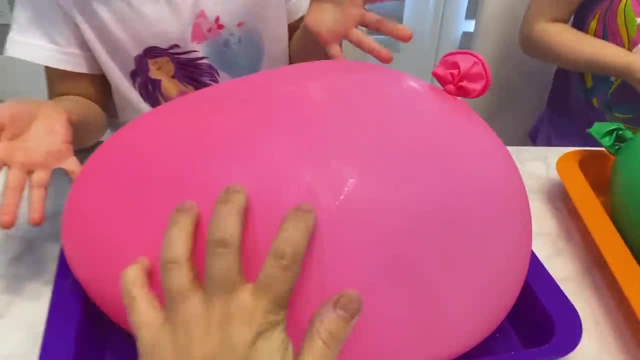 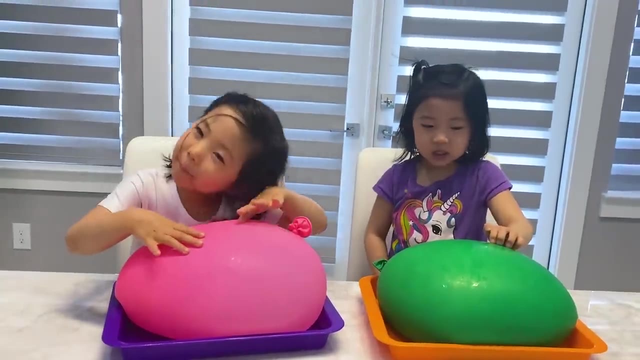 What's inside? Ice Ice that Mommy filled up. Do you see it? It's thick, Yeah, it's super hard. I think mine is a pig. You think it's a pig inside. So, Mommy, also put an animal or an insect. 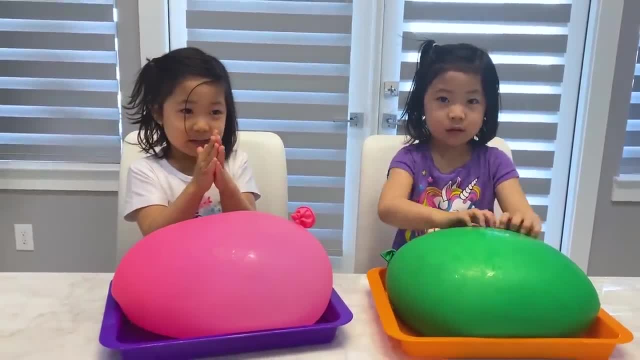 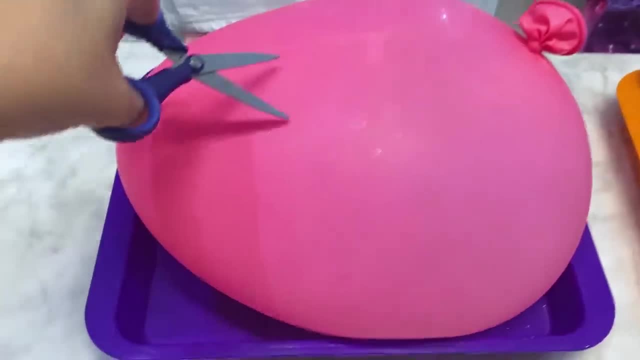 inside. I don't know, We're going to find out. You ready to open it? Are you going to open it? Yeah, I forgot. You ready to open it and free the animal and save the animal? Yeah, So I'm going to cut a little bit Grown up. 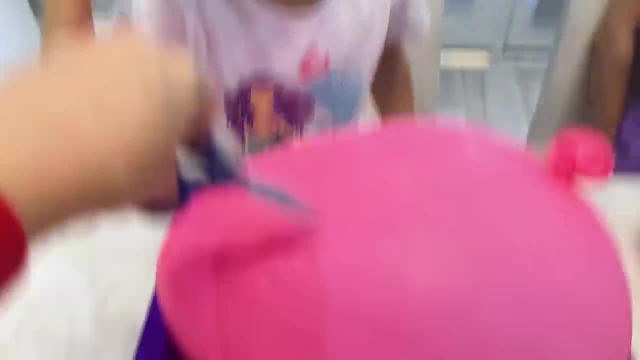 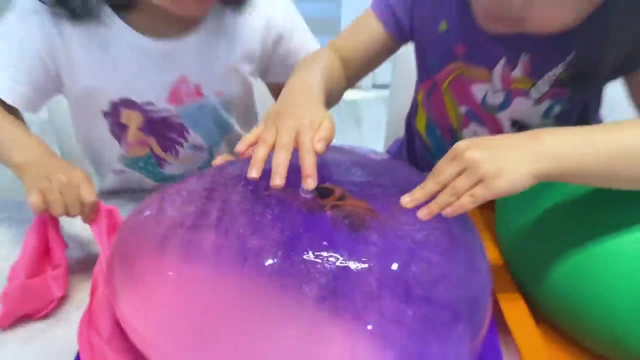 only Thanks, Mommy. Yeah, of course, Kay. Whoa, Mommy, you can't open it, Whoa. So there it is. What animal do you see? A spider, An ant, An ant or a spider Ant Ant, That's. 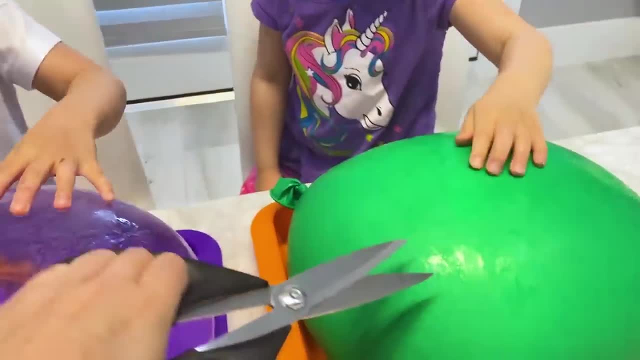 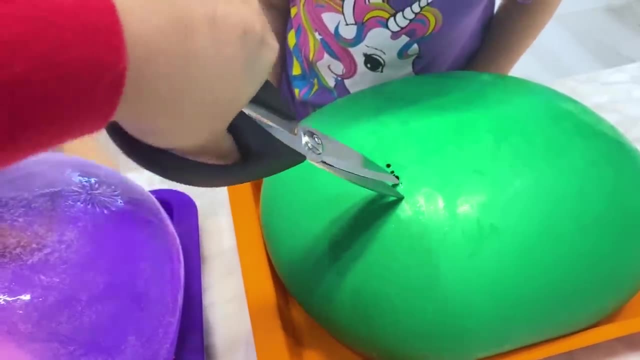 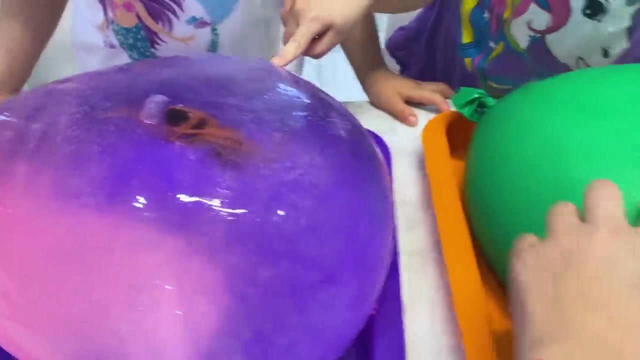 really cool. Mommy, help me. You kissed it. Emma's turn Hand away, please. So grown up. only, There's a little crack here. What is that? Food coloring? Yeah, I actually. yeah, I did put food coloring, so that's why you see the color. Kay, I kept it clear, but, Emma, I put. 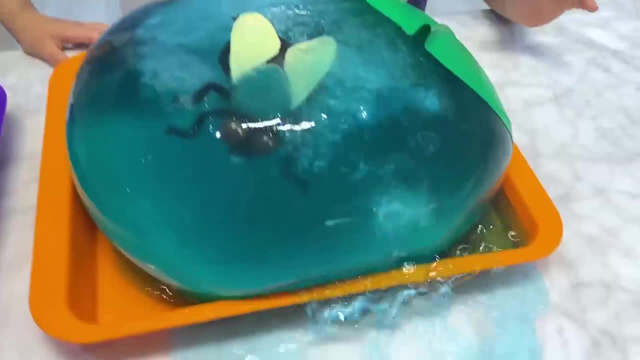 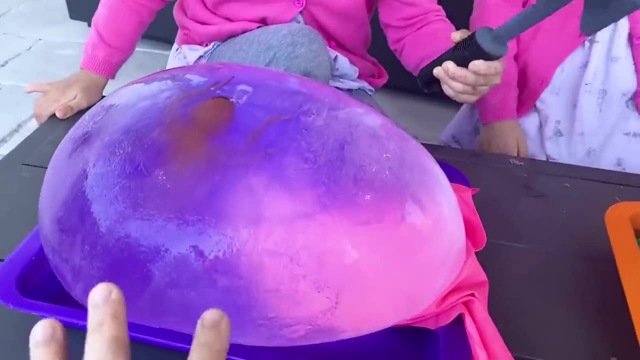 food coloring. Whoa, Whoa, it's dripping already. Oh no, There's a leak. Hey guys, we're on five now. So we're on five because we don't want to make a mess inside. So there's Kay. 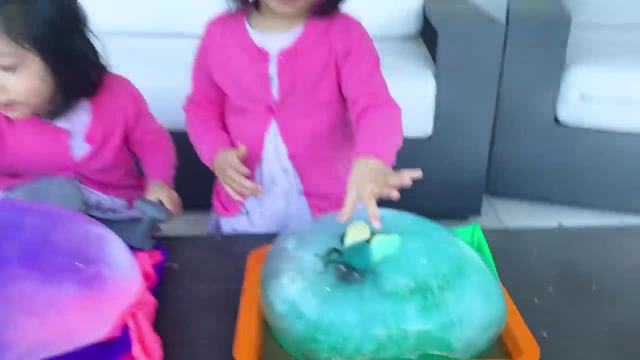 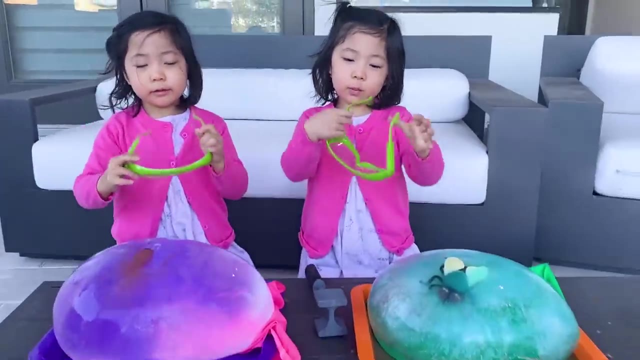 and here's Emma. What animal is yours, Emma? Mine is a pig. Okay, so before we begin, we're going to need some goggles, just in case. right, We don't want to go in her eyes, That's right. There you go, And before Emma Kay does the experiment. 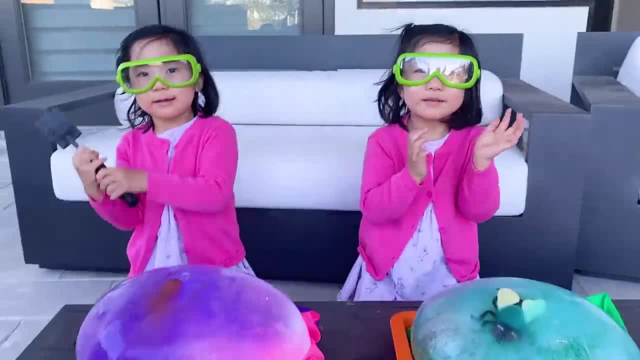 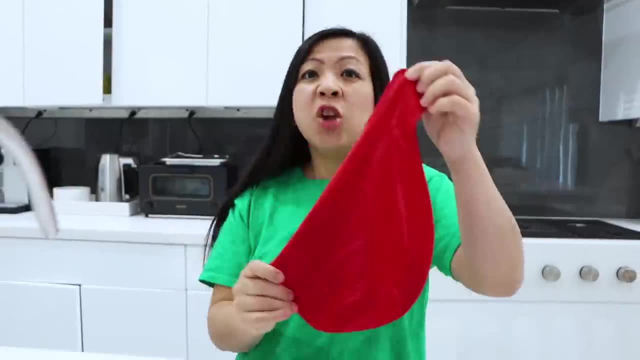 let me show you guys how I did it. Okay, you want to know? Yeah, Roll the clip, Roll the clip. Okay, so first thing, you're going to need to make your own giant ice balloon. is a balloon. You can use a small one or you can use a big one. Here's a clip from when. 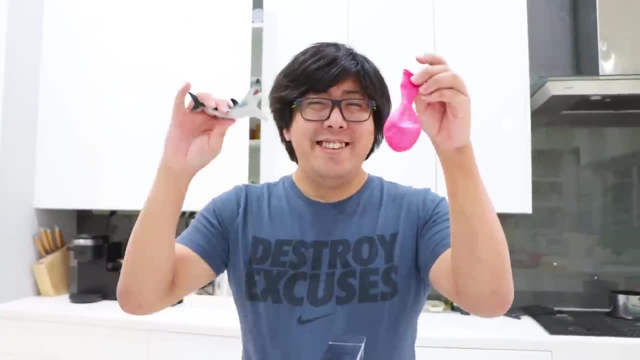 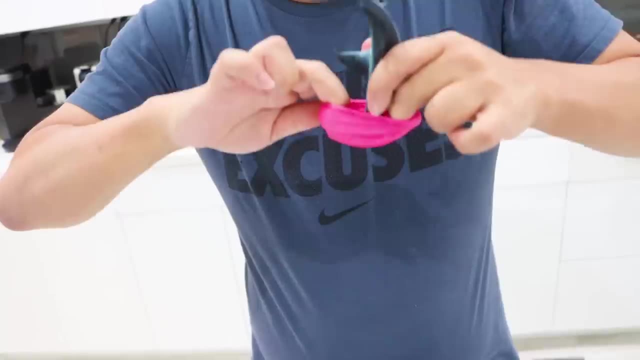 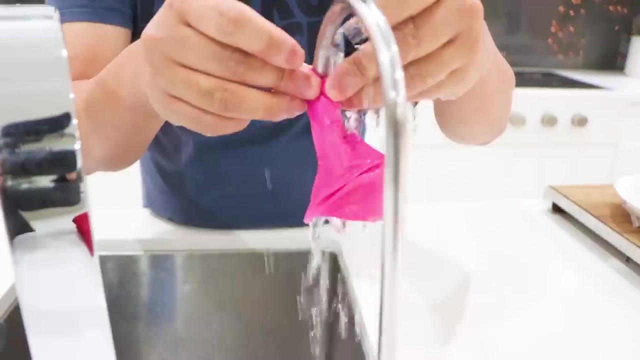 Ryan's daddy made it for us: First grab a balloon, Then get your favorite toy. Carefully, put the toy inside the balloon, Did I mention. carefully, Once the toy is inside, fill the balloon with water. Oopsie, Carefully not to splash water everywhere. 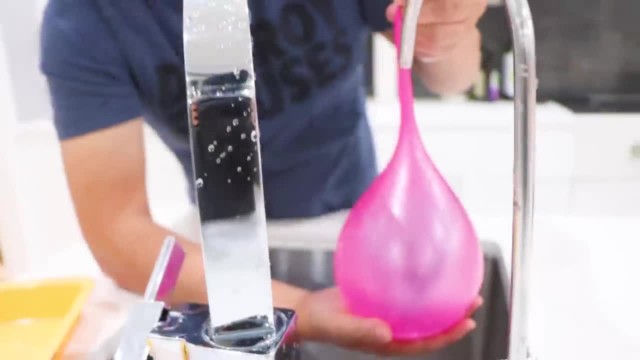 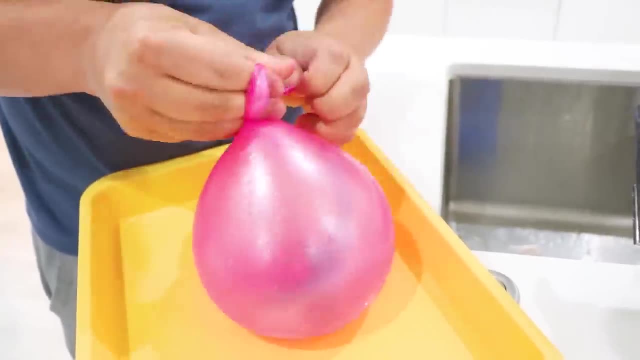 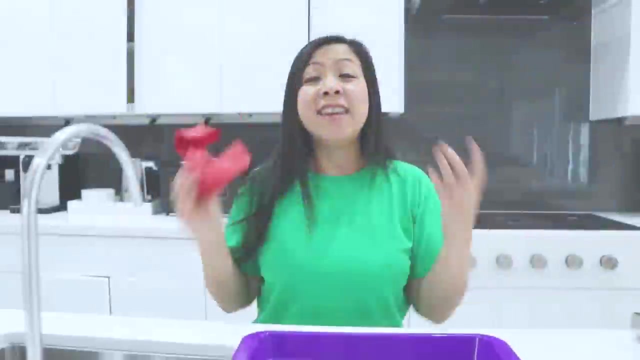 The balloon will get bigger and bigger. Then remove it and put it on the tray. Next, tie the balloon so the water won't spill out everywhere. Next, put the balloon in the freezer until the water inside becomes ice. Now here's for the bigger version. So this: 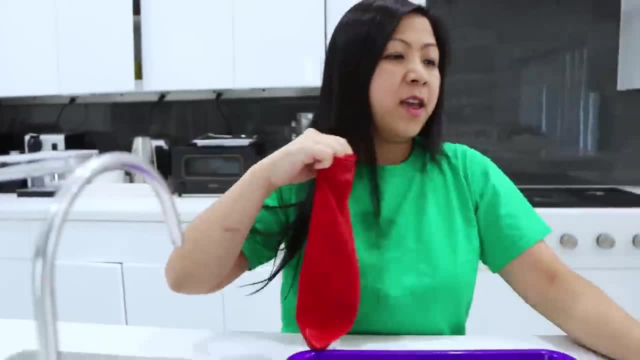 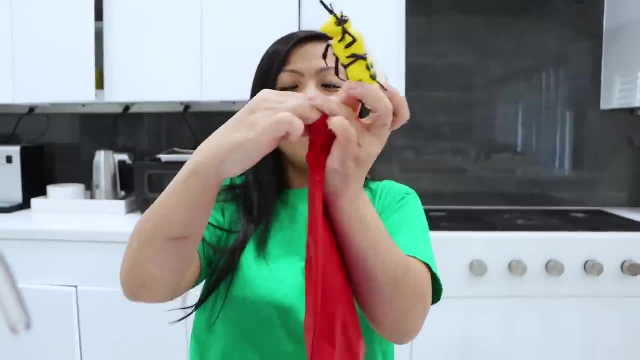 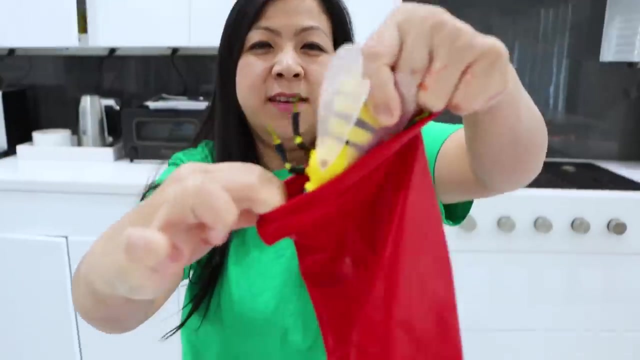 is a giant size balloon, Okay, and then you can put any animals in it, but this one I'm going to use a little bee. All right, in you go bee, Don't worry, We'll rescue you later. okay, Let's go in, Go Tight. Okay, there you go, And then just fill it with. 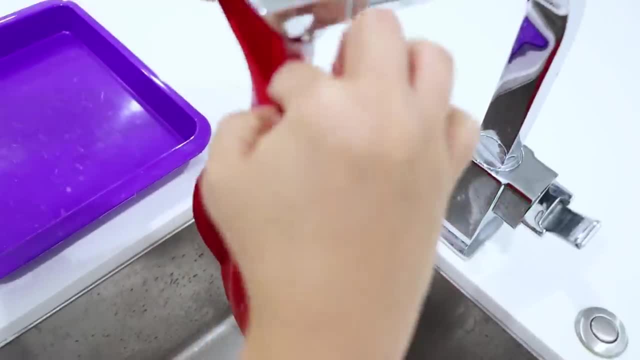 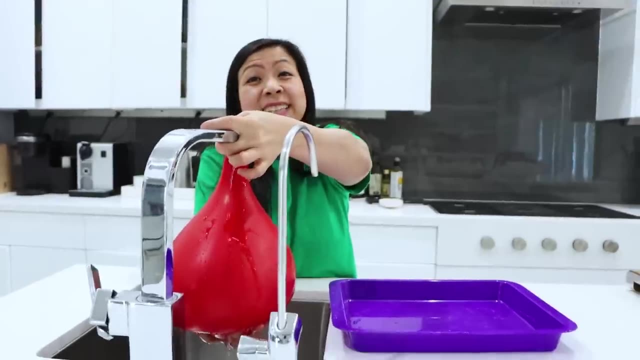 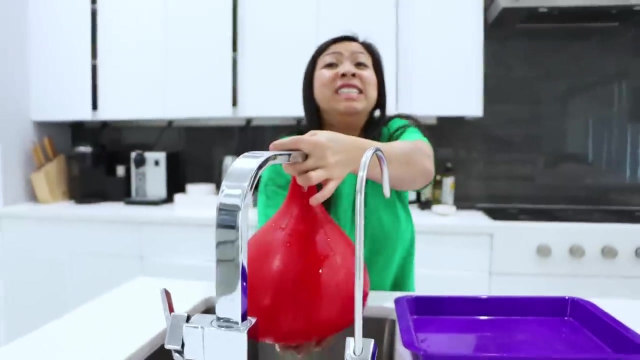 water. That's it. Fill it with water Super easy. Okay, guys, So I fill up water and you have to be very careful because it gets heavy. Look, It's like super heavy and bouncy. I don't have the strong muscles- Super, super heavy, but I'm going to try to make it a lot. 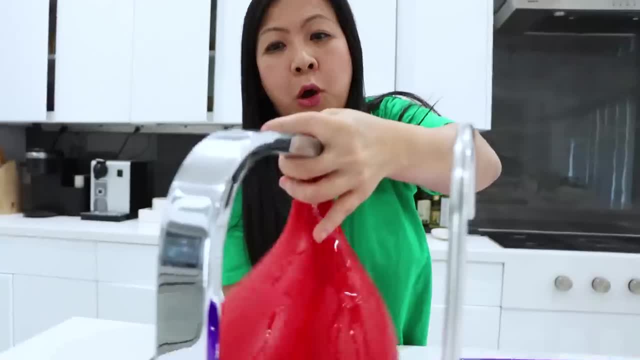 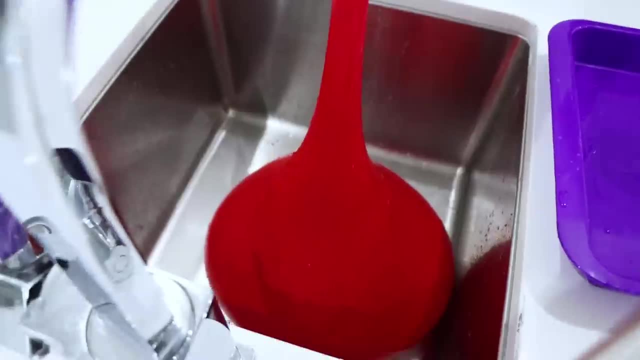 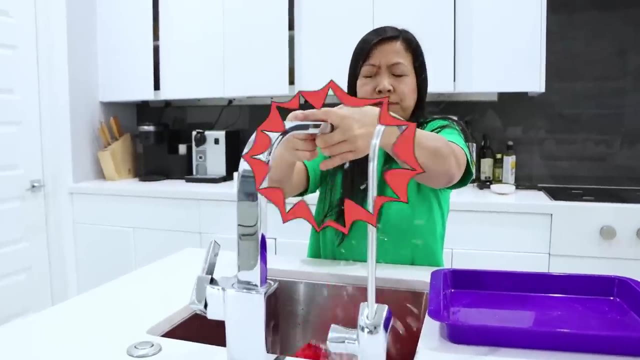 bigger. Okay, not a lot, but like a little bigger, Okay. Whoa. Look how jiggly it is. Woohoo, Okay, so I can't hold it anymore. Look what's happening. Once you think it's big enough, turn off the water, Untie And then tie your balloon. 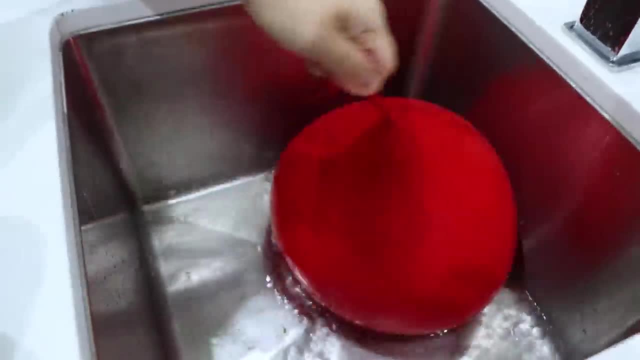 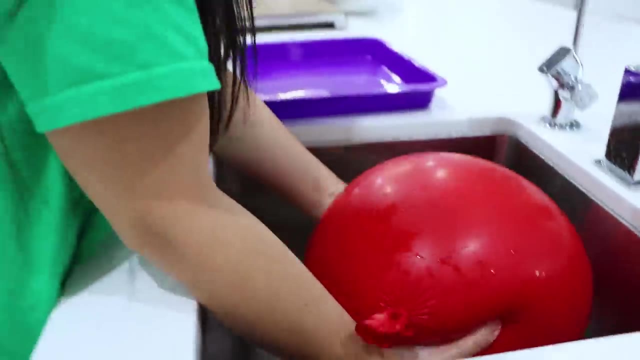 See It's done. Look how wiggly it is. It's so fun. And the bee is somewhere in there, Can you see it? And then, using some strong muscle, parents only. Whoa, This is slippery. Okay, I should have asked Daddy to do this. 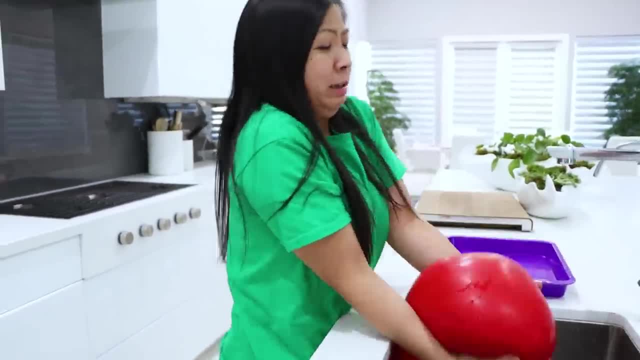 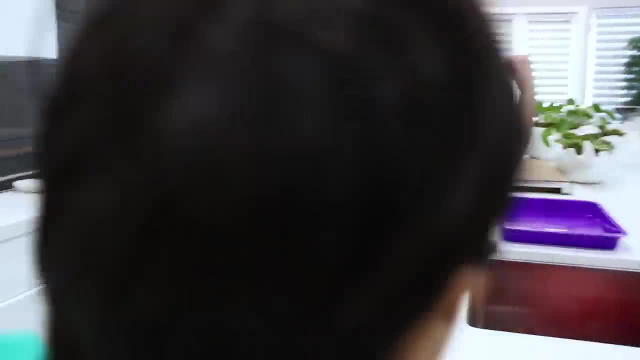 Okay, Okay, I'm using strong muscle. Ahh, I really got this. guys, You want to try? Try? Come on, Ryan's going to try. He thinks he's got stronger muscle than Mommy. That's so jiggly. 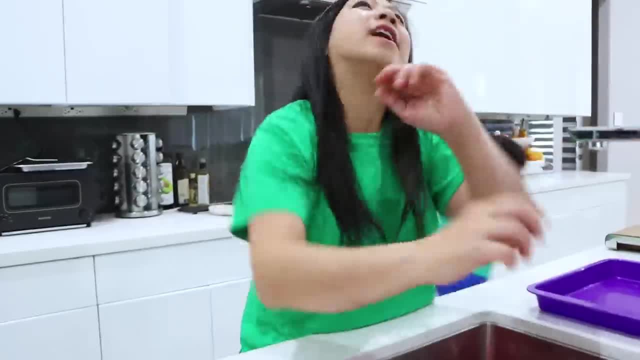 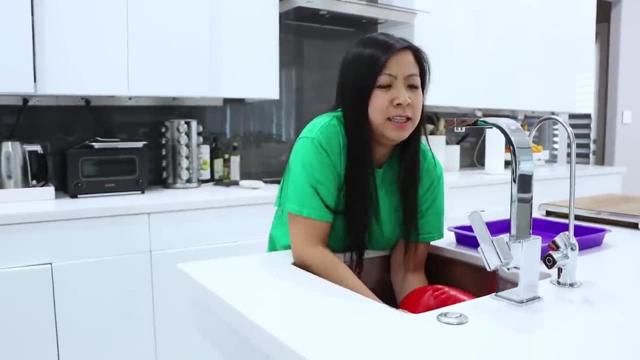 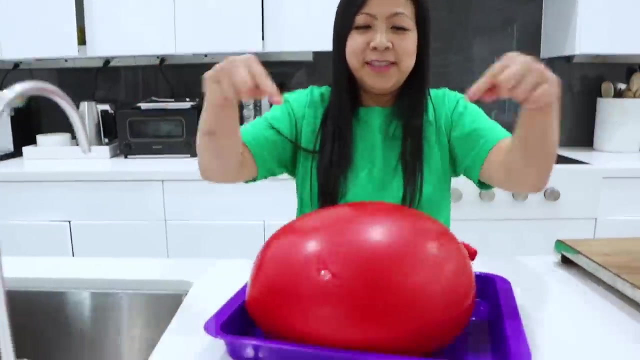 Okay, Mommy will pull it. Ok, Mommy got this. I've been working out for this past two days. Okay, ready, Lift, lift, lift, lift, See, See, And then just put it on a tray. Okay, Look, how fun this is. It's like. 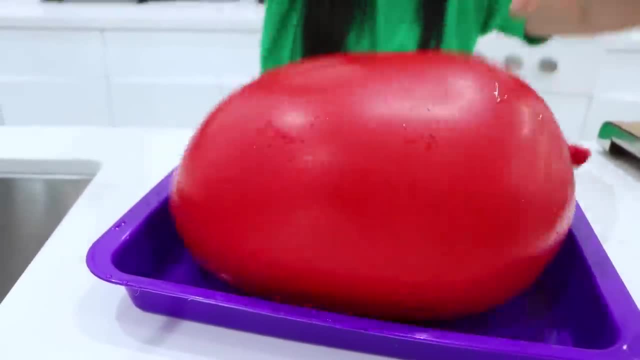 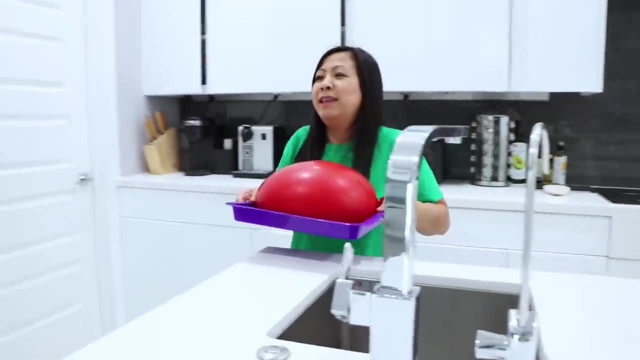 a wobble bubble. Is that what it's called? Wobble bubble, Wobble bubble, And that's all you do. You just pick it up and, Ryan, can you please open the fridge for mommy, because it's super, super heavy, Thank you. And then just open the freezer. Open the freezer and 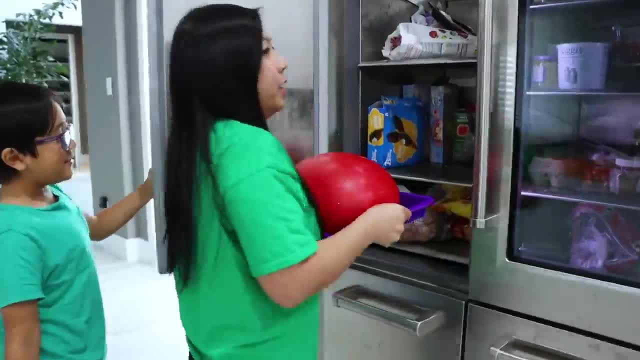 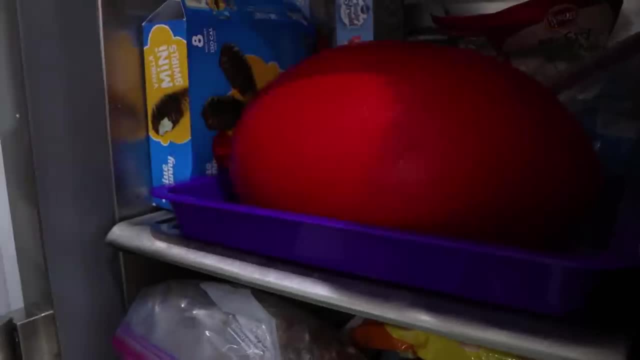 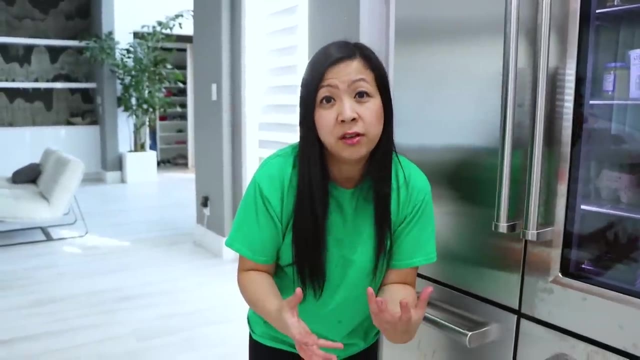 then, carefully, carefully, boom, boom, boom, boom, put it into the freezer. There it is Alright. Good luck with that. Let it sit overnight. So if you don't let it sit overnight long enough, there could be water in there still, Okay. So that's what happened to us. But the 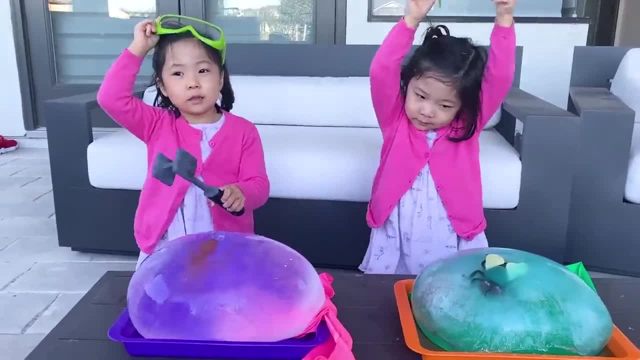 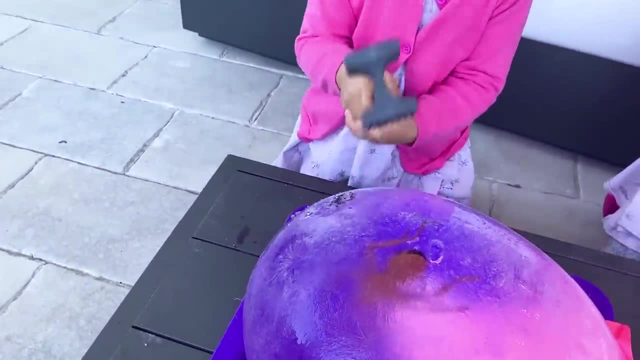 longer you wait, the better. Okay, We're back. You guys ready to get started? Yes, Okay, So Kate's going to try first. Let's see. Ooh, It's a little bit hard, huh, And only do this with grownups, right? Whoa, Look what. 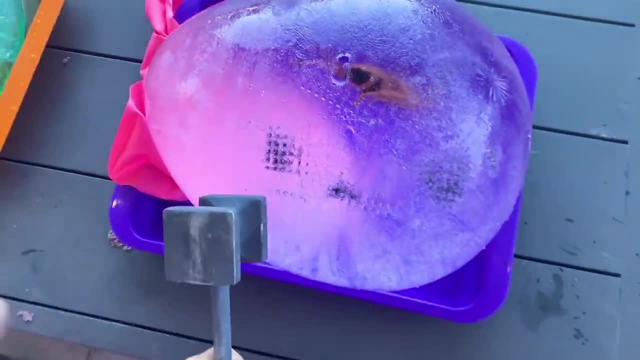 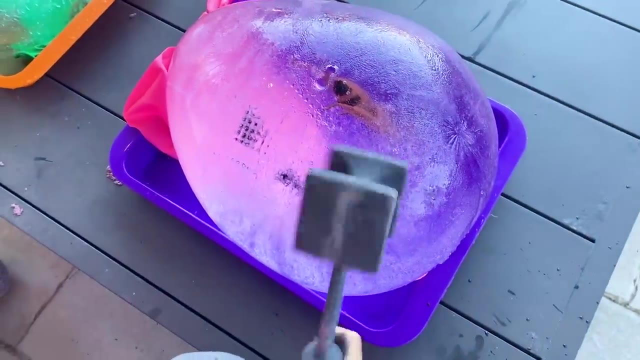 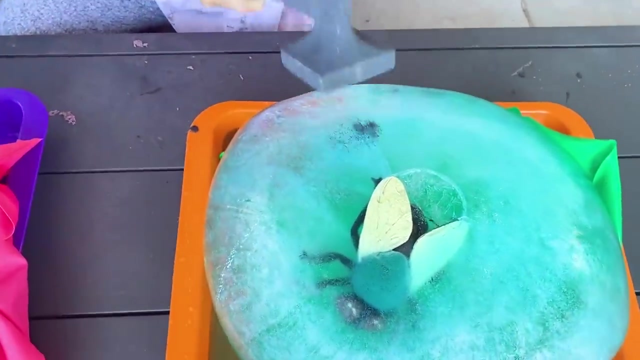 happened when I braked it. Yeah, I think there's a little dirt on the hammer that mommy didn't clean. Sorry, It's okay. Yeah, It's still good. Whoa, Is it working? It works. It works a little bit. huh, Not a lot. Okay, Emma's turn. It's not easy. huh, Oh, Emma, you broke. 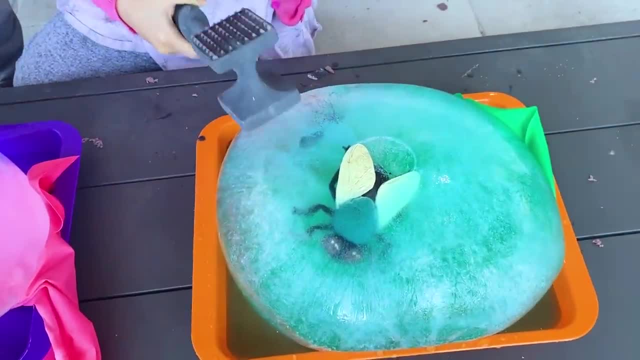 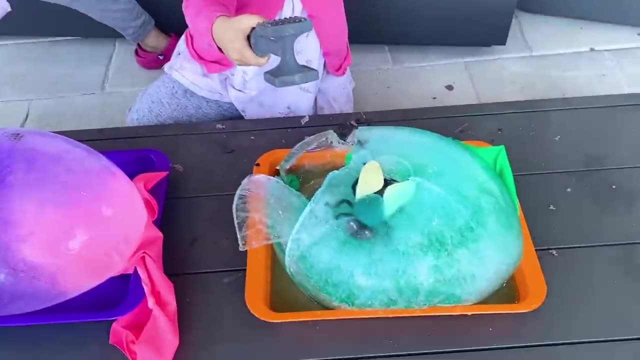 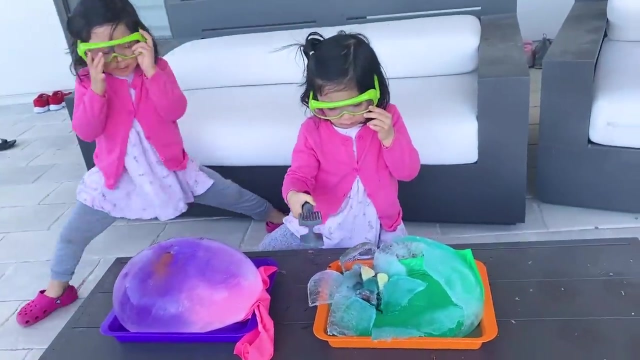 it a little bit Nice, You can do it, Emma, You can do this. You can do this. Whoa Nice. Whoa, Emma, you did it. You freed the fly. You're freeing it. Yay, You can do it. Yay, Emma, you did. 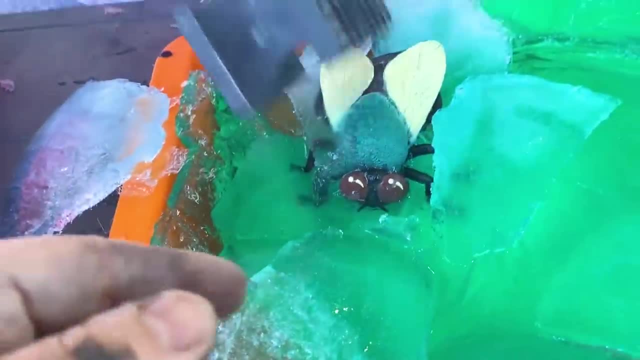 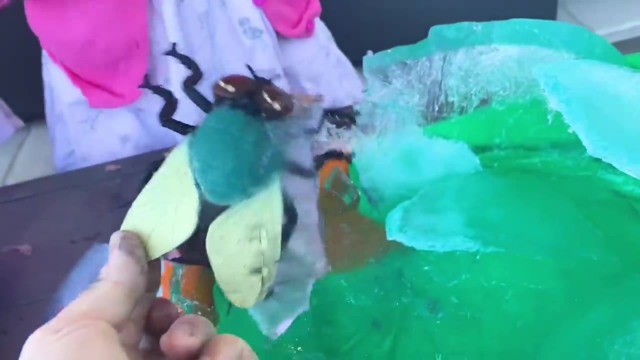 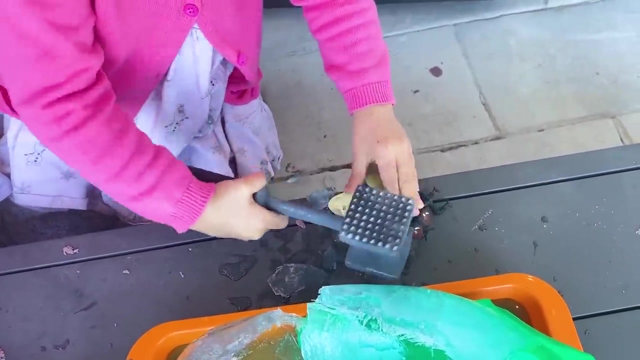 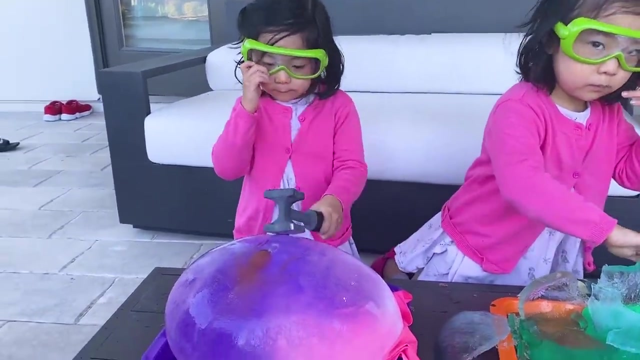 it. Good job, Emma. Oh, look, It's still a little bit left. The fly is almost free, Do you see it? Yeah, look It's a little bit unfree. Yeah, There you go. Nice, You freed the fly, Good job, Okay. Yeah, So Kate turned, but it's a little bit. 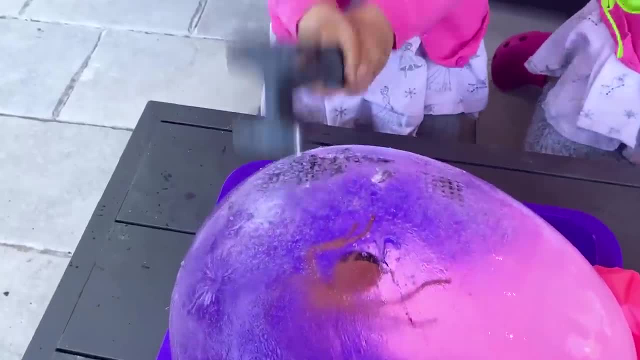 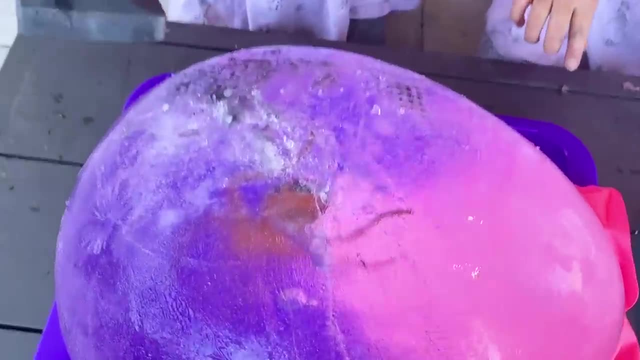 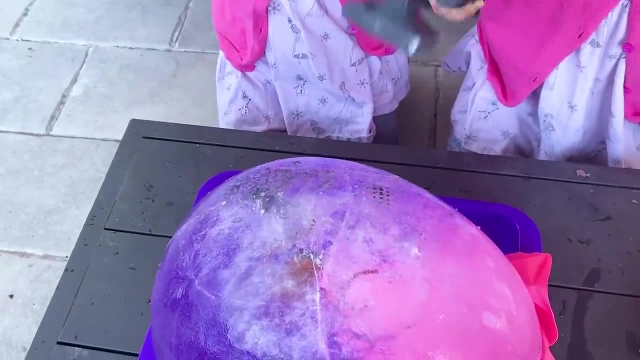 hard, since Kate is a little bit harder, right? Oh look, Whoa, You're doing great. Look, It's almost cracking. Look, Oh look, Look, You can see water inside. Can you see the water? Okay, Emma's taking over and helping Kate, Whoa.